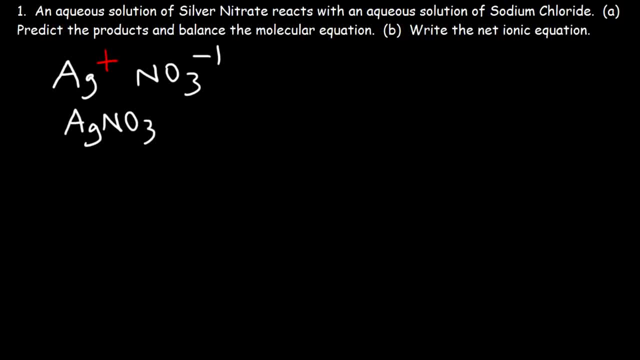 write silver nitrate as AgNO3.. Sodium has a plus one charge- It's found in group 1a of the periodic table- and chloride has a minus one charge, So you can write the two as NaCl. Now to predict the products, you need to realize that. 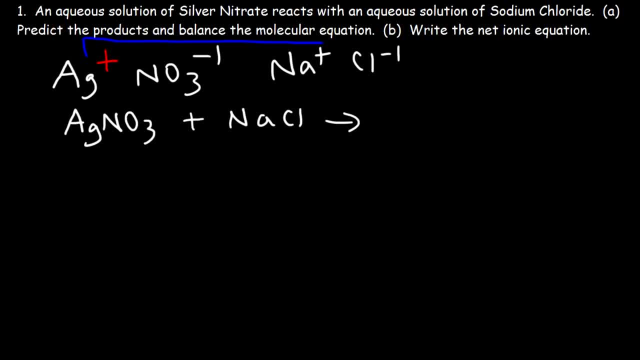 silver is going to pair up with chloride and sodium is going to pair up with nitrate. It's a double replacement reaction. Always put the positively charged ion first and then write the negatively charged ion next to it. When Ag and Cl pairs up, they're going to combine in the 1 to 1 ratio because the charges are the 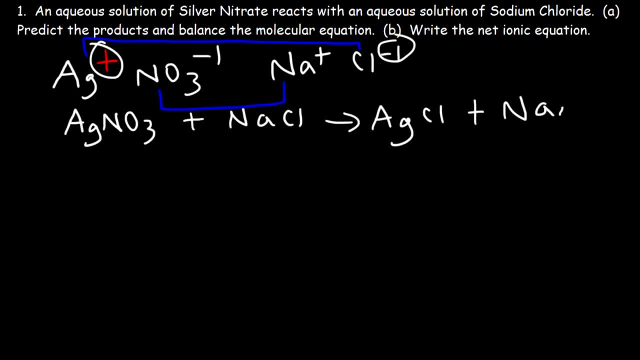 same, and the same is true for Na and NO3.. So this is the balanced molecular equation, and all we need to do is write the phases. So this is aqueous. aqueous Nitrates are always soluble, so this is aqueous. it dissolves in water. Silver. 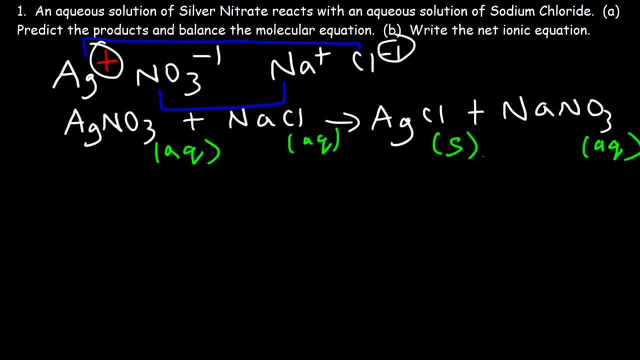 chloride is insoluble. Chlorides are usually soluble except with silver, lead and mercury. Now the next thing that we need to do is we need to write the total ionic equation. So everything that is in the aqueous phase we need to separate into ions, The 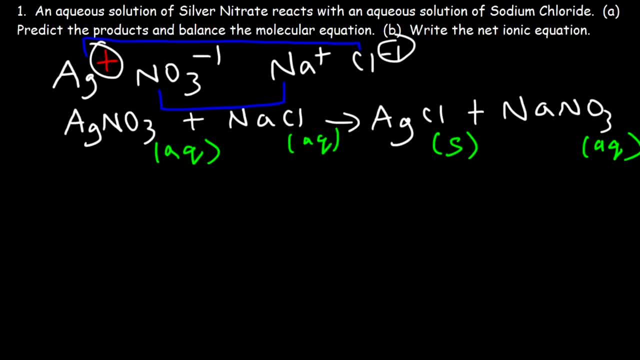 only thing that's going to remain the same is the solid product, silver chloride. Whenever you mix two aqueous solutions and when you get a solid product, this is known as a precipitation reaction. So this is going to be Ag+, which is in. 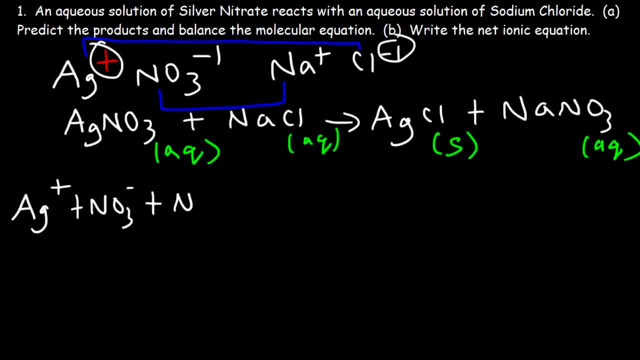 aqueous phase, Plus nitrate, plus Na+, and then we have Cl- AgCl is going to stay the same, so this is the only solid that we have. Everything else is in the aqueous phase. And then sodium nitrate. we can write it as Na+ and NO3- So this is the 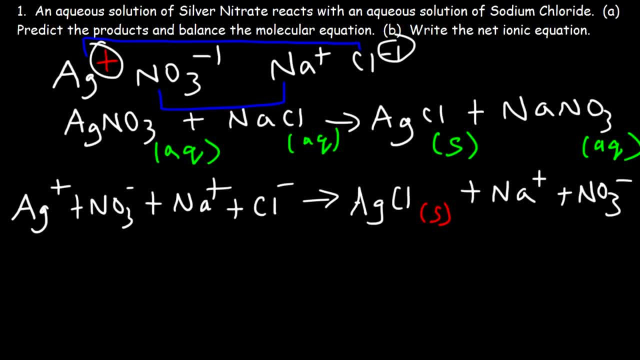 total ionic equation. Now what we need to do is eliminate the spectra ions. Sodium is a spectra ion because it's the same on both sides. The spectra ions: they don't really participate in the reaction, They basically watch it. They're just spectra's. 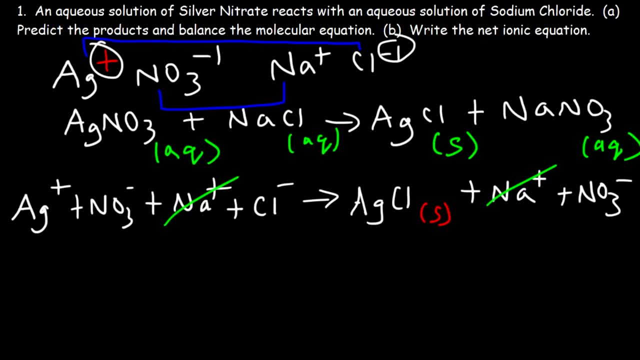 And the other ion that's found on both sides of the reaction is nitrate, so that's another spectra ion. So what you have left over is the net ionic equation, So Ag+, which is in the aqueous phase, plus Cl-. 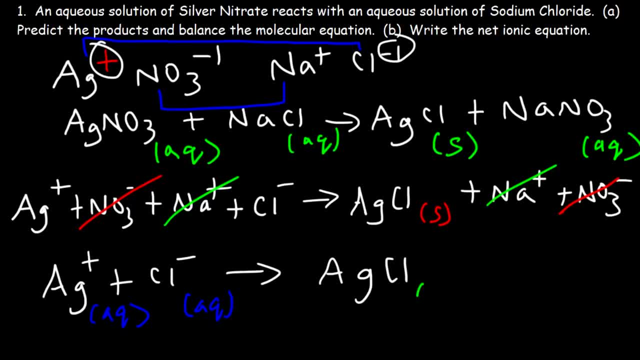 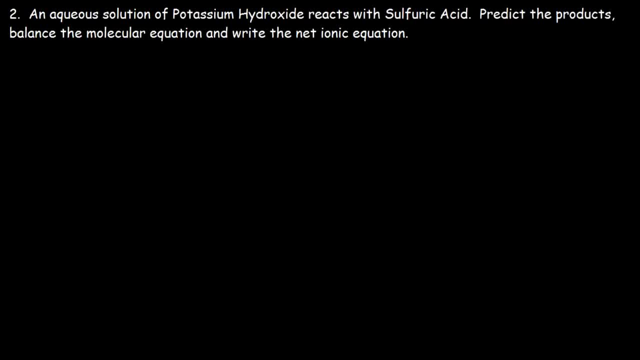 will produce silver chloride, which is in the solid phase. So that's a precipitation reaction. Number two, an aqueous solution of potassium hydroxide reacts with sulfuric acid. Potassium is an alkali metal found in group one, so it has a plus one charge. Hydroxide is a polyatomic ion. 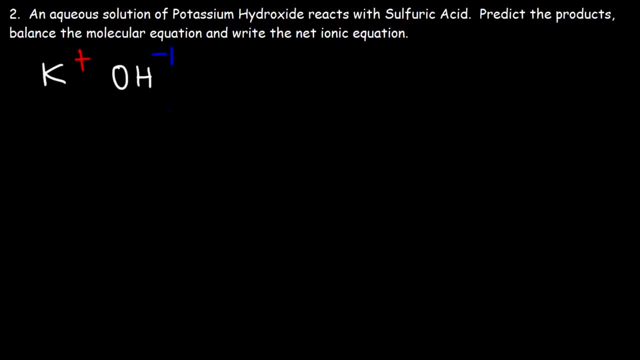 with a negative one charge. So because the charges are the same, we can simply write it as KOH, And the solution is aqueous, so it's dissolved in water. Sulfuric acid. Sulfuric acid comes from the polyatomic ion sulfate. 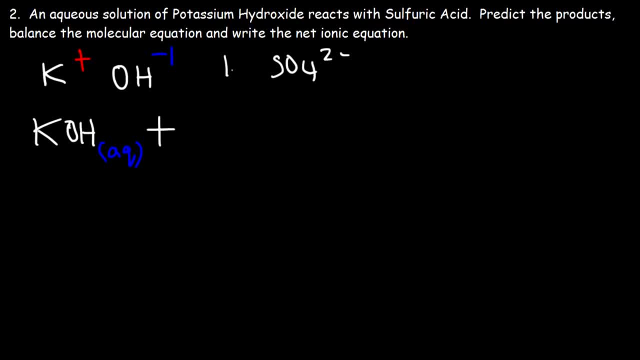 which has a minus two charge, And because it's an acid, it's going to have an H plus in front of it. So if you use the crisscross method, it's H2, SO4.. So that's the formula for sulfuric acid. 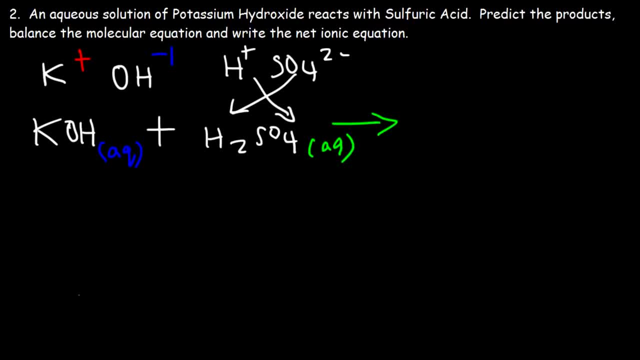 So what are the products of this reaction? The positively charged metal ion, K, is going to pair up with the negatively charged sulfate ion. When K plus and sulfate get together, they're going to form potassium sulfate, which is K2,, SO4, 1, or just SO4. 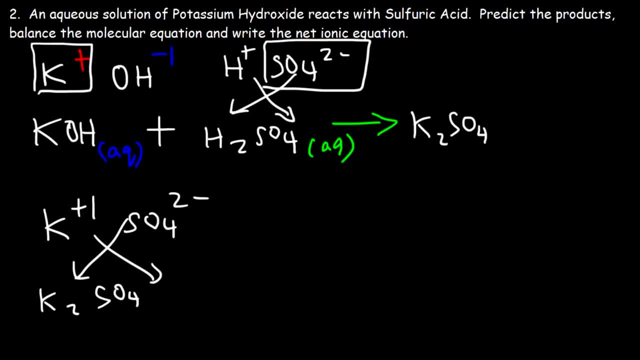 That's going to be one of the products Now, all of the group one: metal cations like sodium and potassium. they're always soluble. So potassium sulfate is soluble. The other two, H and OH, they're going to pair up. 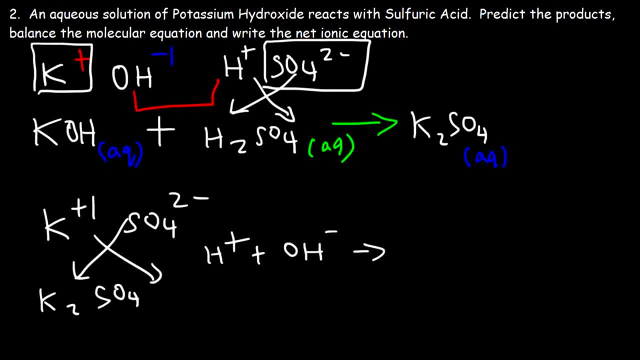 Whenever you have hydrogen ions reacting with hydroxide ions, they will combine to create liquid water. So those are the products of the reaction. So what we have here is an acid-base neutralization reaction. Potassium hydroxide is a base. 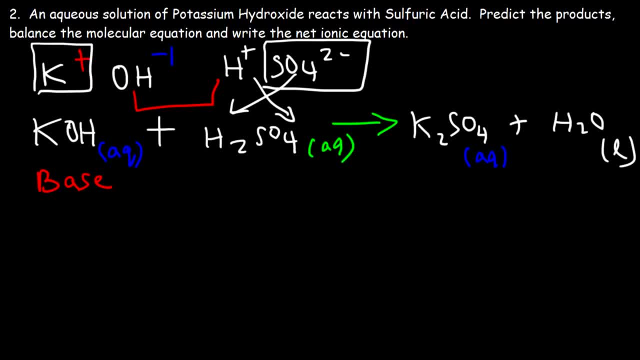 All metal hydroxides are bases. Sulfuric acid: well, that's an acid. Whenever you mix a strong acid and a strong base, it's going to produce salt and water. The pH comes to be about seven. It neutralizes. 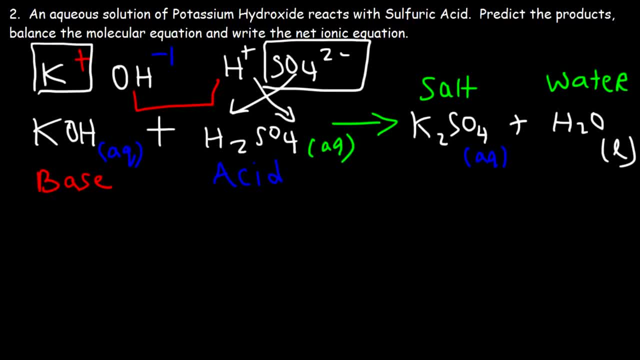 The pH of acetic solutions is less than seven. For basic solutions it's greater than seven. When you get salt and water, the pH is going to be about seven. Now what we need to do is balance the reaction. So how can we do so? 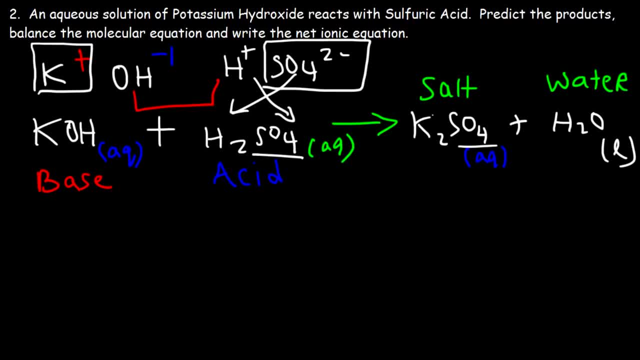 We have one sulfate ion. We have two potassium atoms on the right, So that means we've got to put a two in front of KOH. Now notice that this will. This means that we have two hydroxide ions and two H+. 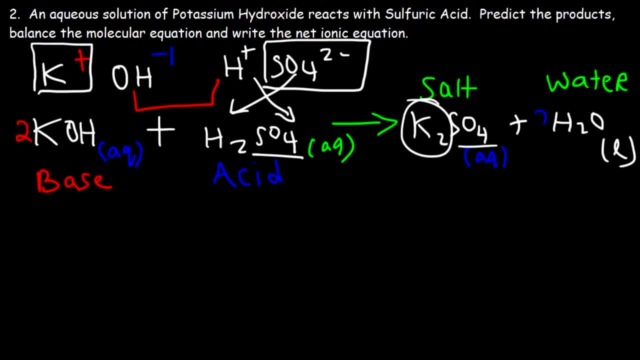 Therefore we need two water molecules For every hydrogen ion and hydroxide ion that combines, one water molecule is produced. So if two hydroxide ions combine with two hydrogen ions, it's going to create two water molecules. If you count the number of hydrogen, oxygen and potassium atoms, you should see that they're the same on both sides. 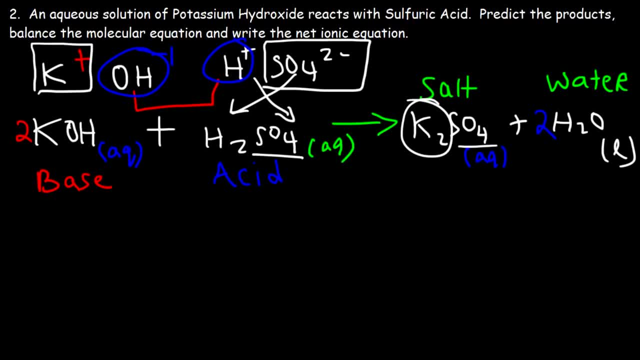 We have two potassium atoms On both sides, one sulfur atom, A total of six oxygen atoms, Four in sulfuric acid, Two in KOH. Here we have four and another two, And we have a total of four hydrogen atoms on both sides. 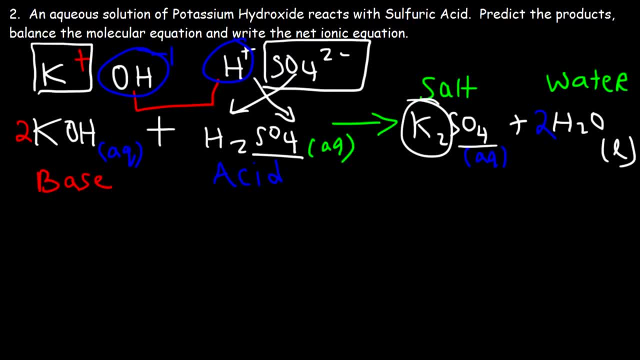 So the reaction is completely balanced. So now we need to write the total ionic equation. So everything that is in an aqueous phase we're going to separate into ions. So let's start with KOH. We have two potassium ions and two hydroxide ions. 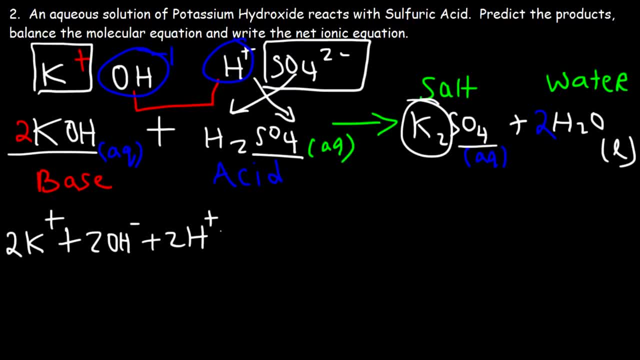 In sulfuric acid, we have two hydrogen ions and one sulfate ion. In potassium sulfate, we have two potassium ions and a sulfate ion. Now, water is not in the aqueous phase, It's a liquid, So we can't separate it. 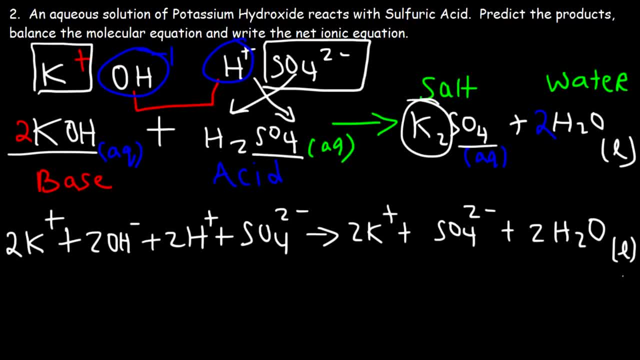 We have to leave it the same way. Our next step is to identify the spectator ions, Which ions look exactly the same on both sides of the reaction. So we have potassium And also sulfate. Those are the spectator ions. So the net ionic equation is 2H+ plus 2OH- yields two water molecules. 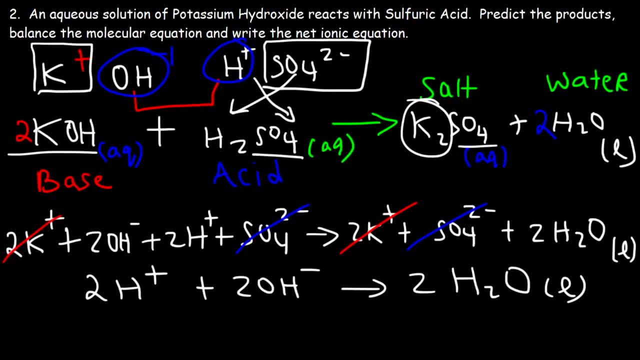 However, because we have a 2 as the coefficient for every species in this reaction, we should divide everything by 2.. So it's going to be H+, which is in the aqueous phase, plus OH- and that's going to produce liquid water. 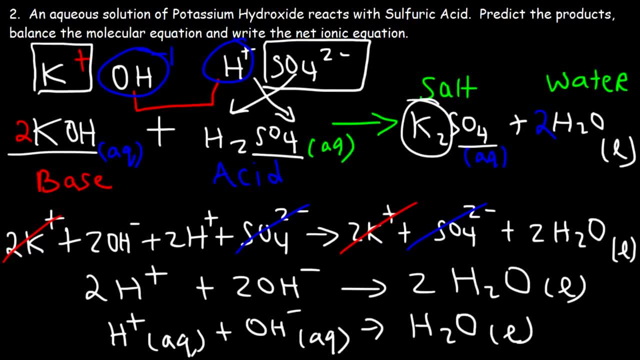 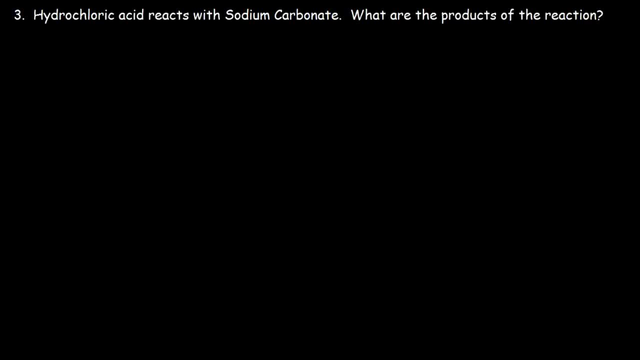 So that's the net. That's the net ionic equation And this is the balanced molecular equation. Hydrochloric acid reacts with sodium carbonate. What are the products of this reaction? Hydrochloric acid is HDL. I think that's just something you should know. 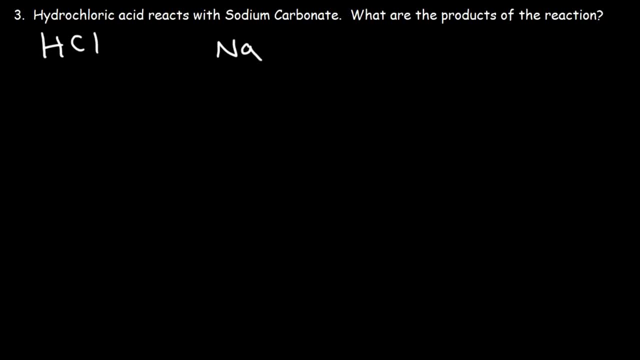 Sodium carbonate. We know that sodium has a plus one charge, since it's a group. one metal cation Carbonate is CO3 2-. So, using the that criss-cross method, the formula for sodium carbonate is going to be Na2CO3.. 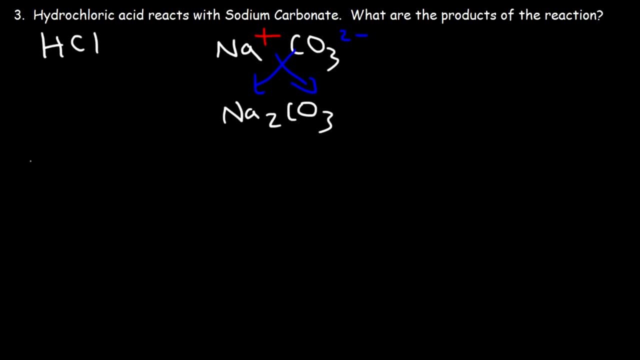 So, therefore, what we have is HDL plus Na2CO3. And let's go ahead and predict the products of this reaction, And typically you could assume that this is going to be in the aqueous solution, unless specified otherwise. I guess this could be a solid placed in hydrochloric acid solution. 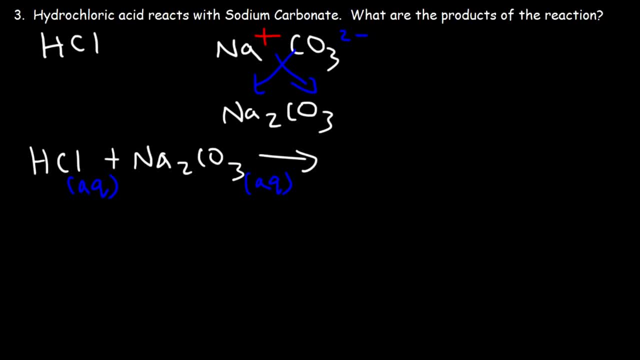 but let's assume it's in the aqueous solution. So now Na is going to pair up with Cl. Na has a plus one charge, Cl has a minus one charge. These two will combine in a one-to-one ratio to produce NaCl. 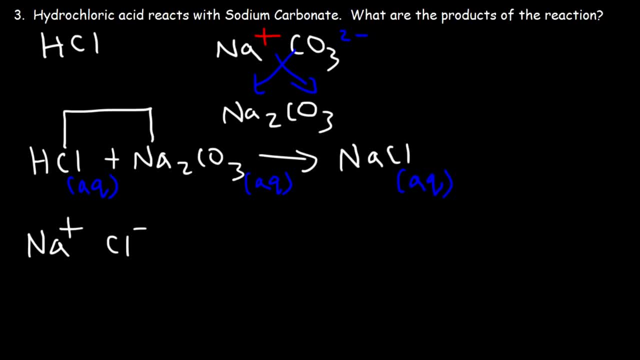 Sodium chloride is soluble. Alkyl metals in group one are always soluble. Now what about the other product? We get a pair of H and CO3.. H has a plus one charge, Carbonate has a minus two charge. So this is going to combine in a two-to-one ratio. 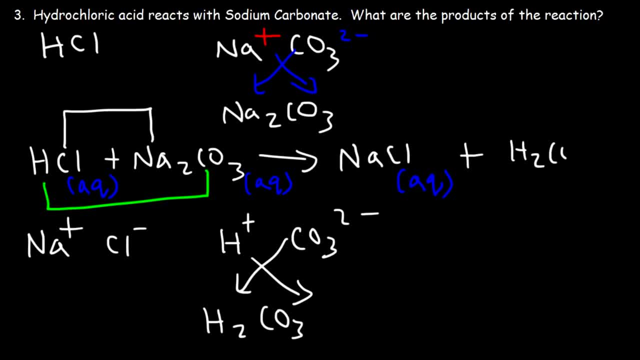 We're going to get H2CO3, carbonic acid. Carbonic acid, like most other acids, can dissolve in water. It's in an aqueous phase. Now, looking at this reaction, everything is in an aqueous phase. 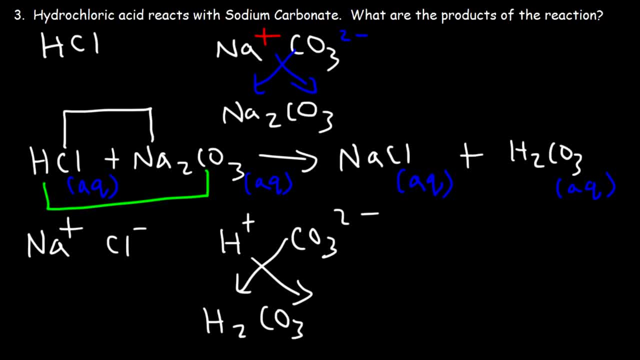 No liquids or solids were formed. This would indicate that no reaction has taken place. However, this particular situation is different. Carbonic acid will decompose into liquid water and gaseous carbon dioxide. The driving force for this reaction is the evolution of a gas. 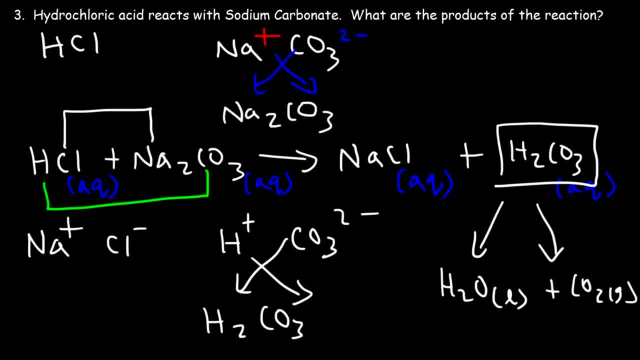 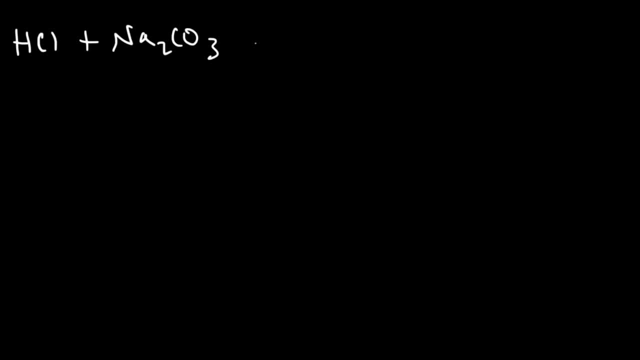 This is a gas evolution reaction. So therefore, what we now have is this reaction: HCl plus sodium chloride Carbonate produces sodium chloride, liquid water and gaseous carbon dioxide. So the first three substances are in the aqueous phase. 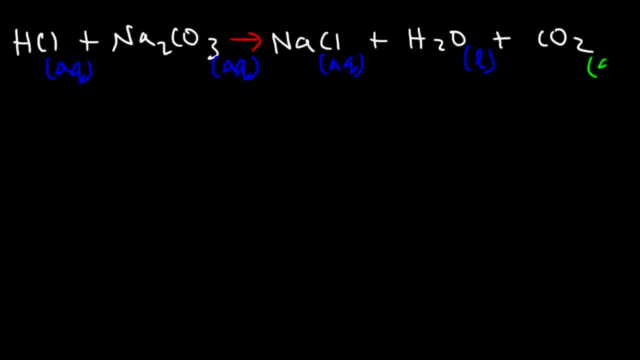 Water is in the liquid phase And this is a gas And if you look at the reaction, it's not balanced. yet We have two sodium atoms on the left side, so we've got to put a 2 in front of NaCl. 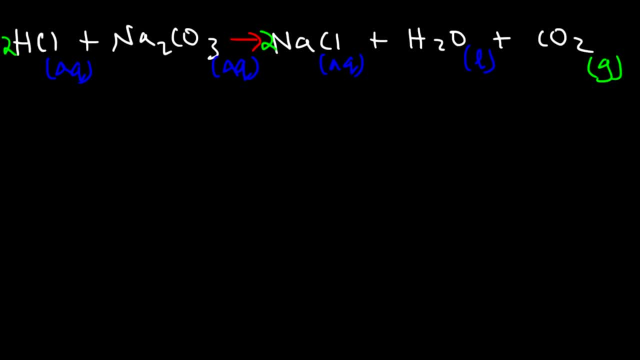 And we have two hydrogens on the right. so we need a 2 in front of HCl And now the reaction is balanced: We have two hydrogens, three oxygens, one carbon atom and two sodium atoms on both sides. 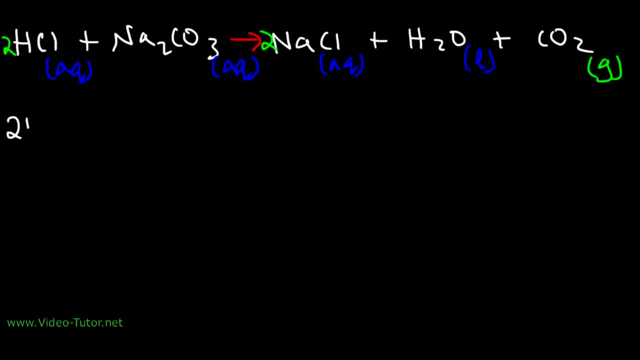 So now we can write the total ionic equation, which is 2H plus 2Cl, minus two sodium ions and one carbonate ion. On the right side we have two Na plus ions, two chloride ions, And we can't change liquid water or gaseous CO2.. 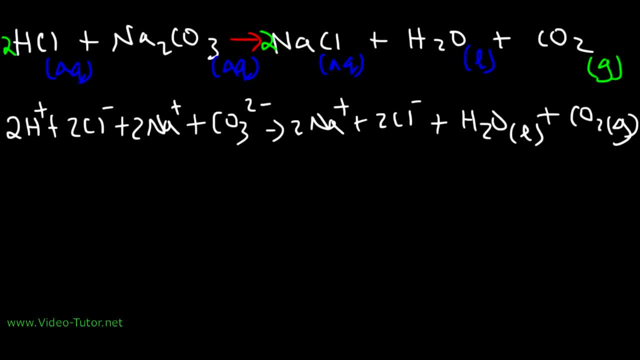 The only thing that we can split up into ions are those in the aqueous phase. So next we need to eliminate the specks of ions, which include sodium and chloride, because they're exactly the same on both sides. So the net ionic reaction is 2H plus in the aqueous phase.